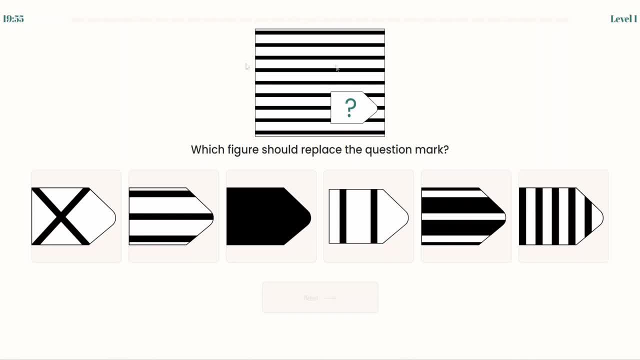 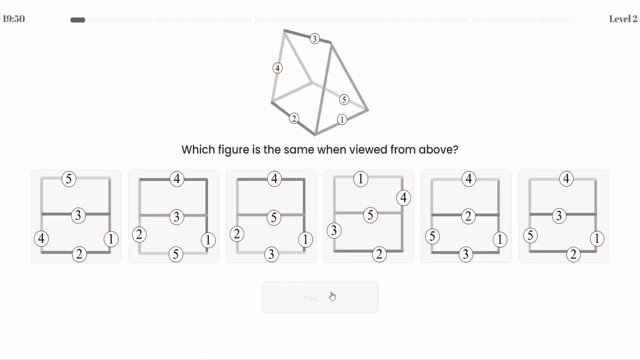 Which figure should replace the question mark? So we have a striped horizontal pattern. Two is correct. Hi, this is me from the future. I just wanted to say that in the top right corner there is a level. Each time you answer a puzzle correct, you level up. And each time you answer. 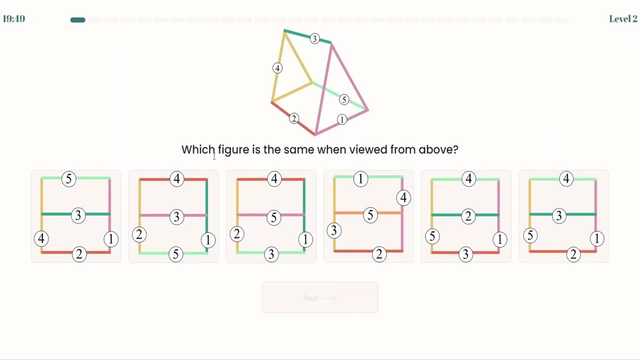 a puzzle incorrect. you level down Which figure is the same when viewed from above. So we have: three is cyan and in the middle it's either one or six. The difference between one and six is that five is this light blue color, And we see that five is this light blue color, So one is. 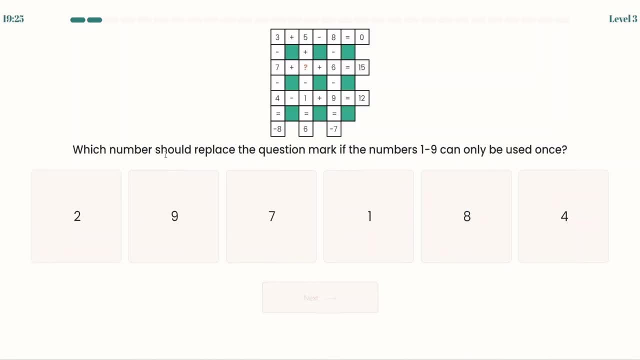 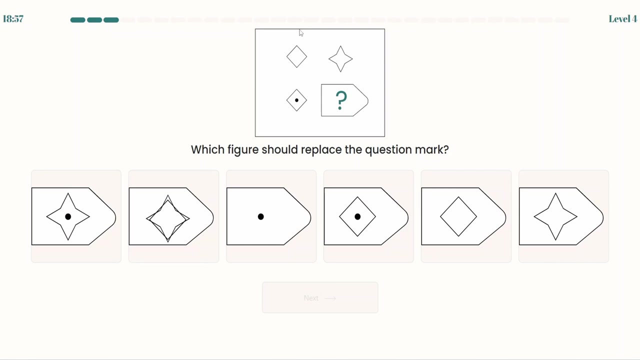 correct Which number should replace the question mark If the numbers 129 can only be used once. so five plus question mark minus one equals six. five minus one is for, So the question mark should be two, because for plus two is six. It looks like the only difference between this column is the dot in the middle. So I expect a star. 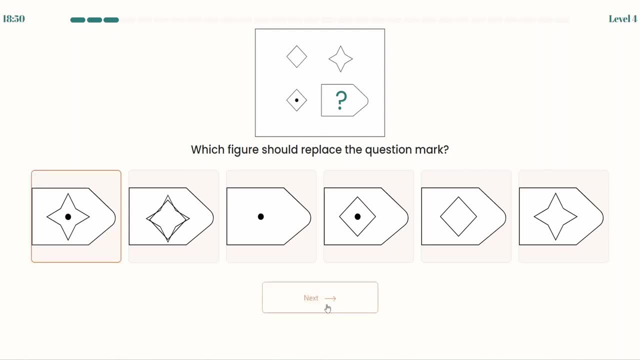 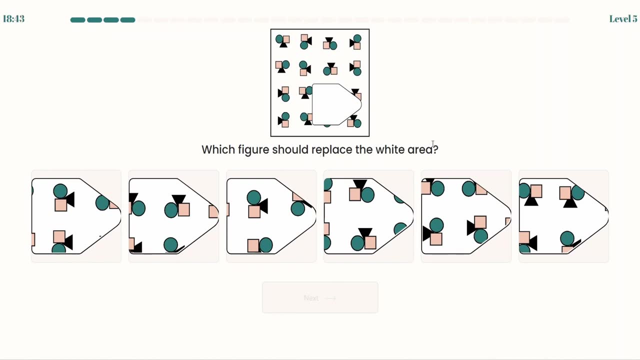 with a dot in the middle, one is correct. Which figure should replace the white area? So the first thing I see is that there should be a blue circle on the top right and a bit of a black triangle on the bottom right. So blue circle on top right, blue circle on top right, blue circle on top right. it's. 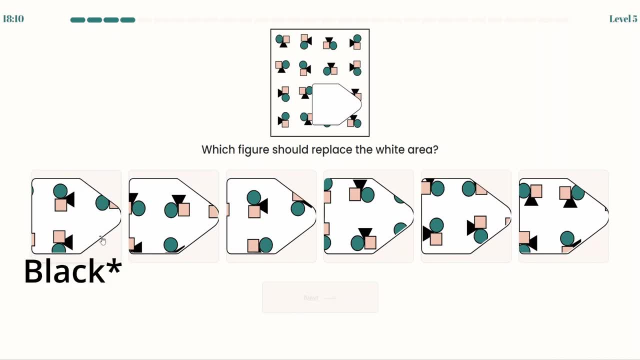 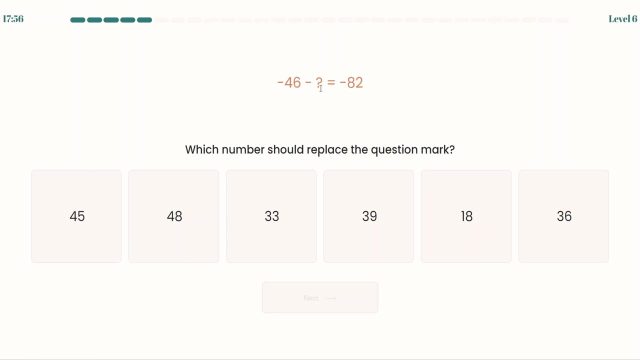 this one Blue circle on top right with some pink blue bottom right and half of a circle on the bottom left. Which number should replace the question mark? Minus 46. minus Question mark equals minus 82. So we just take 82 minus 46 and we get 42 minus 6, that's 36.. 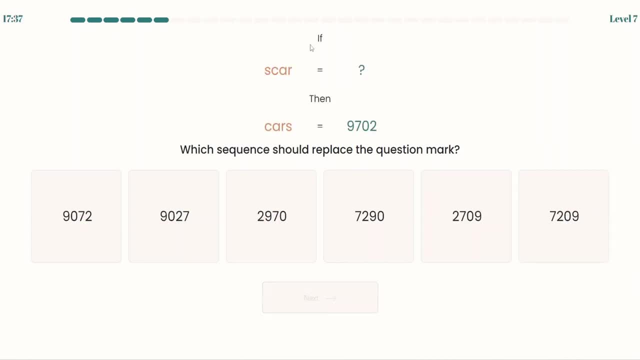 So 36 is correct. If scar equals question mark, then cars equals 9702.. So cars 9,, or I mean the last one, is 2.. So the first digit should be 2.. We have either this or this. 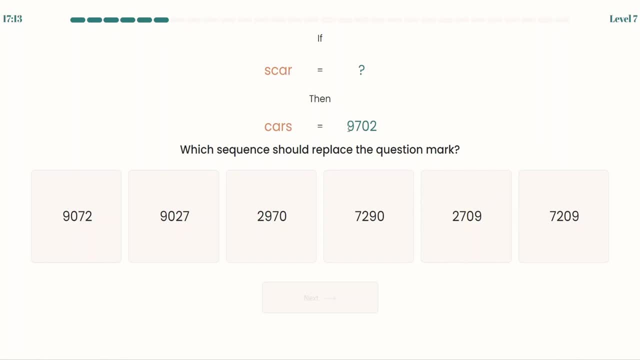 The second digit is C, which is 7.. So the second digit is 72709.. I just wanted to say that I thought about this puzzle wrong. So the second digit should be the first digit of cars, which is 9.. So the correct answer is 2970.. 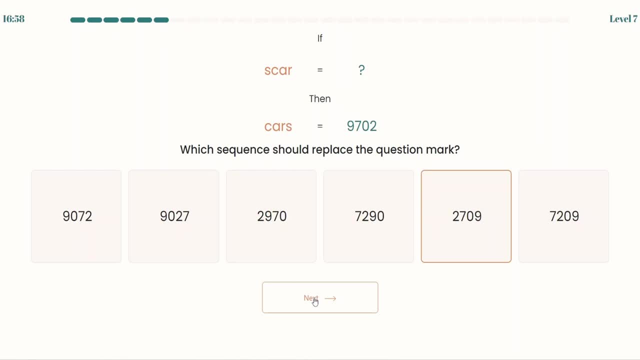 The third answer. The test actually got stuck earlier. I hope it doesn't happen again. I don't know if it's my bad internet or. Oh, there we go. Which three shapes can be combined to create the figure on the left? 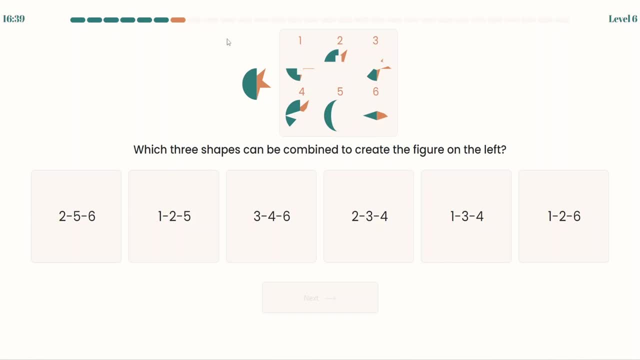 It's not 5.. It's not 5, I think. Wait, is it 5?? It might be. It's not 1 and 2.. So it has to be 4,, 6, and 3? 463.. 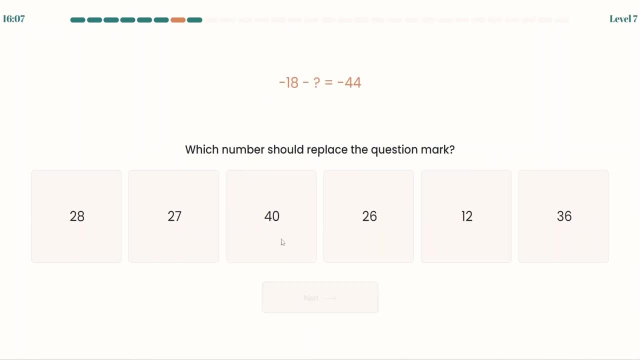 463.. 346.. Okay, Wait, Wait, My last one was wrong. Okay, I need to go back and look at that question and see what I got wrong. Which number should replace the question mark? Minus 18 minus 44, minus question mark. 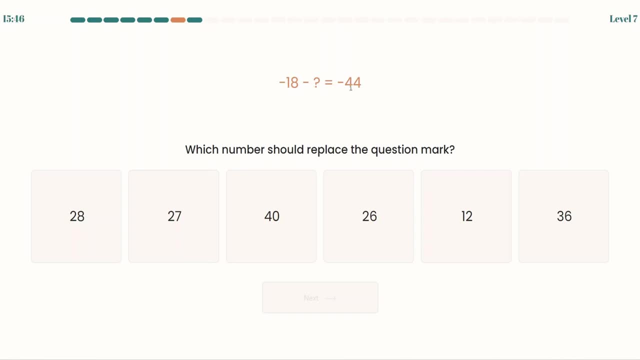 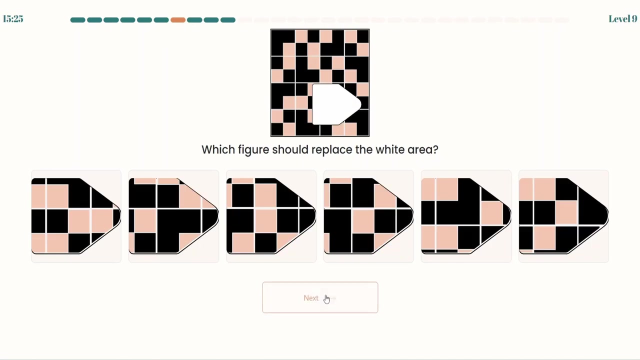 So 44 minus 18.. That's 34 minus 8.. That's 26.. 26 is correct. Okay, So if 2 blue dots is 10 stars, then 1 blue dot is 5 stars. 5 stars is correct. 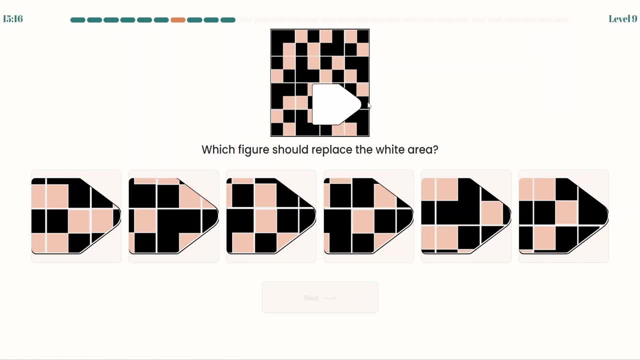 Okay. So I see in the bottom left corner there is this black down, white down black, blue, blue, blue, Black down black and purple right above. I mean pink right above. So black, black, black, pink. 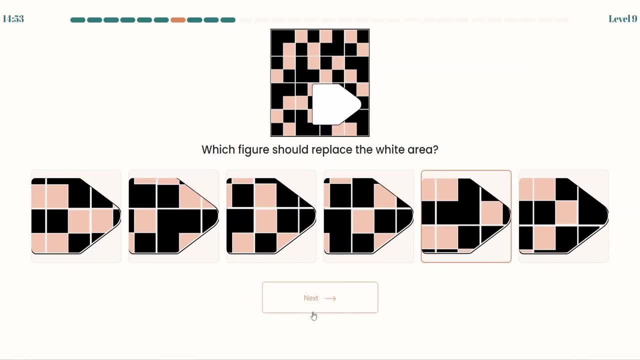 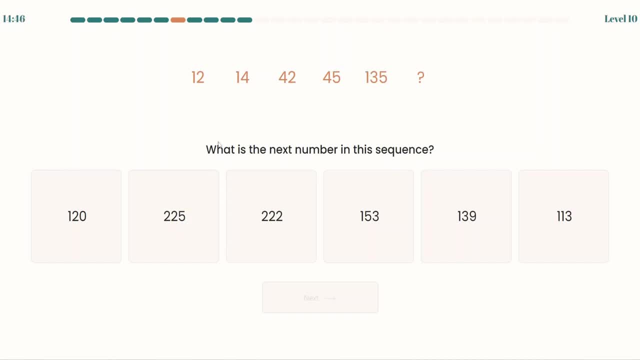 This is the only one that does black, black, pink, So I know that this is correct for a fact. 12,, 14,, 42,, 45,, 135 question mark: What is the next number in the sequence? So plus 2.. 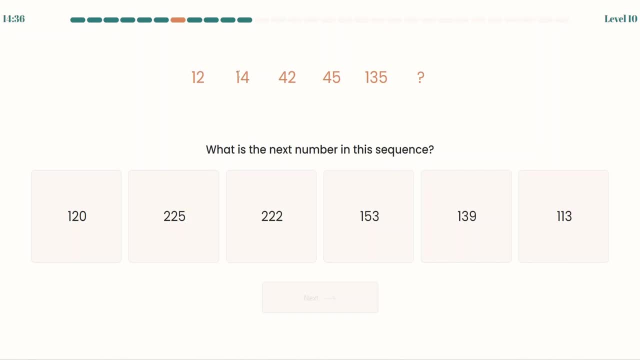 And then, times 3 plus 3, times 3 plus 4,, 139.. Yeah, Okay, So purple equals purple equals red. Okay, So red- I mean squares- is equal to triangles. Squares is the same as triangles. 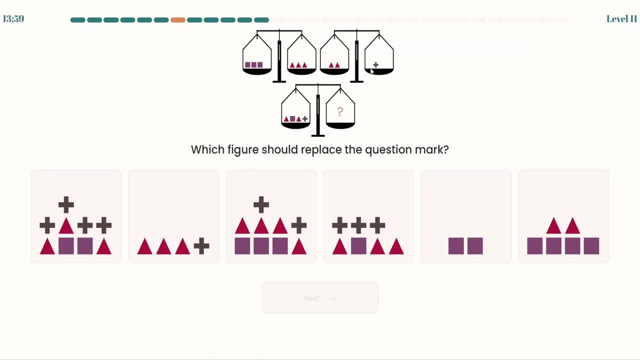 And 2 triangles is 1 plus mark. So 1 plus mark, that means that we can have 5 shapes that are either squares or triangles. So is there any 5 shapes? Nope, There is no 5 shapes, So we can remove 2 of them. 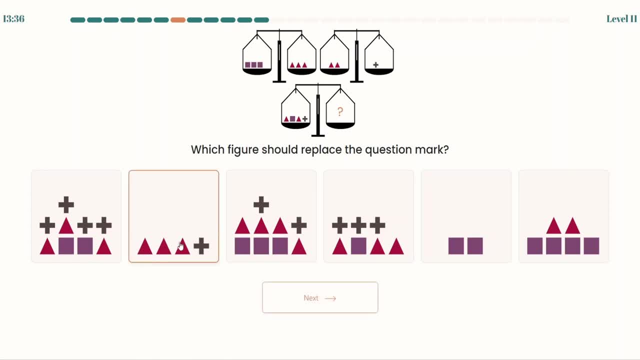 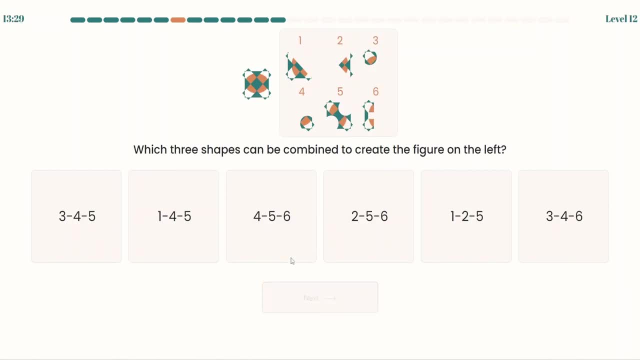 Is there 4 shapes? Yes, Here we have 4 shapes. 3 of them are square triangle and 1 is a plus mark. Which 3 shapes can be combined to create the figure on the left? It's 3. 3.. 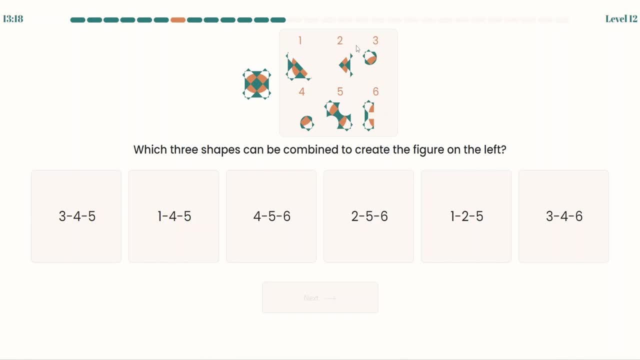 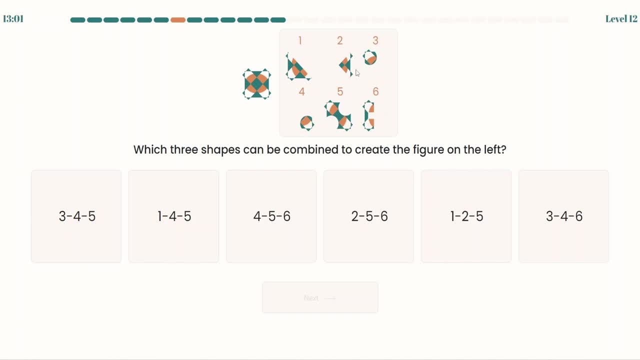 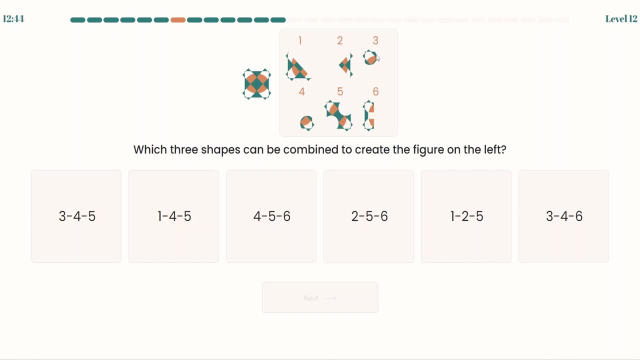 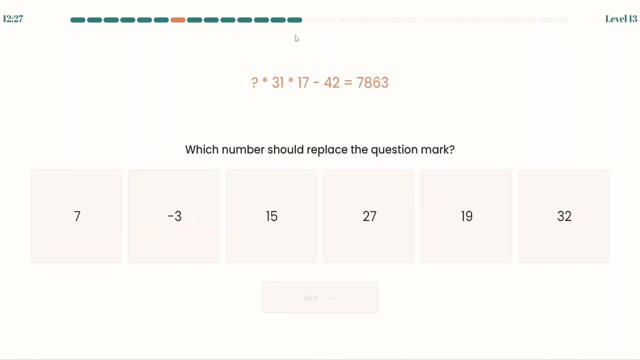 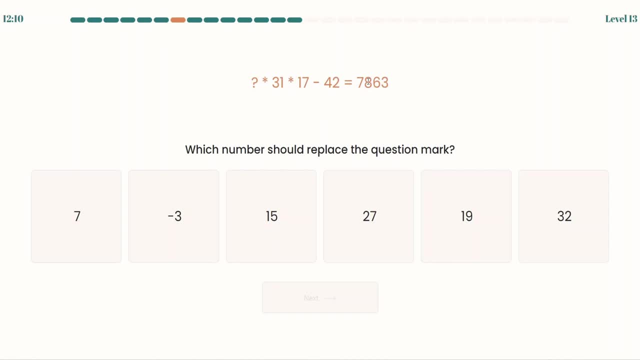 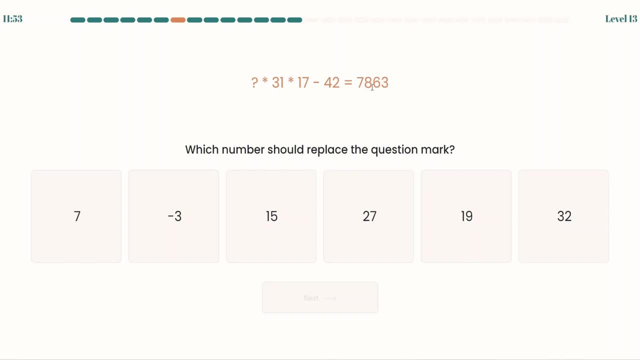 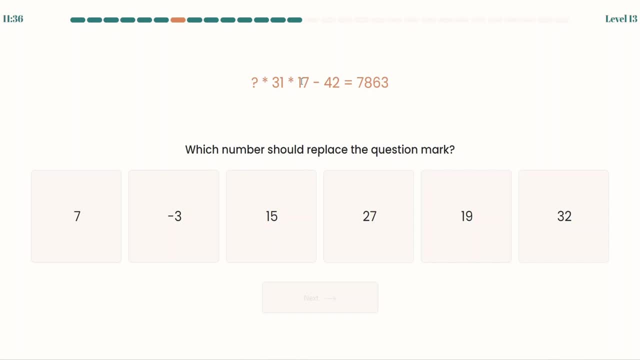 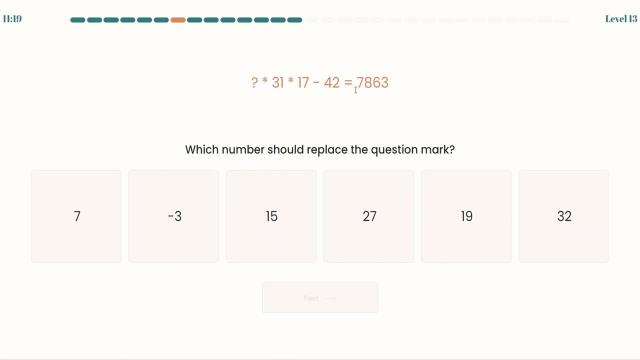 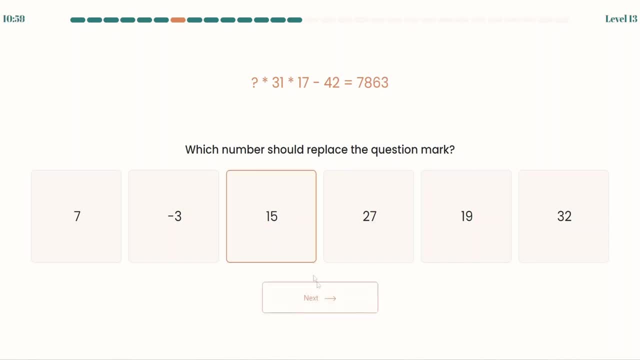 So we go one lower because it's lower and that's higher, so we get 15,. 15 is correct. Okay. so here we have three triangles, here we have two triangles. We eliminate two and we get that two blue. we get that a red is equal to two blue, two. 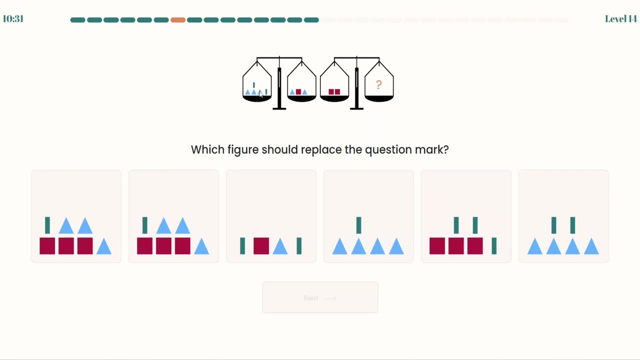 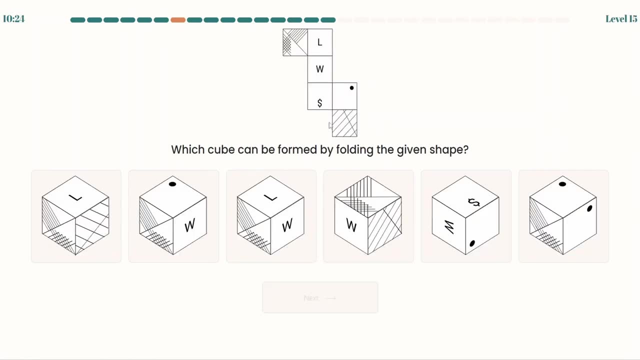 lines plus a triangle. two lines plus a triangle. two lines plus a triangle. okay, this is correct. A red: two lines plus a triangle. Which cube can be formed by folding the given shape? I'm always struggling solving this. I'm thinking maybe one. 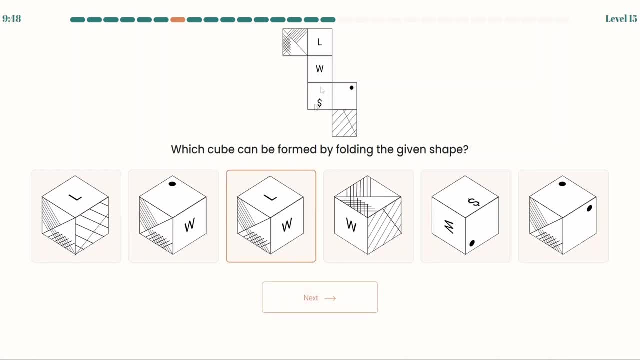 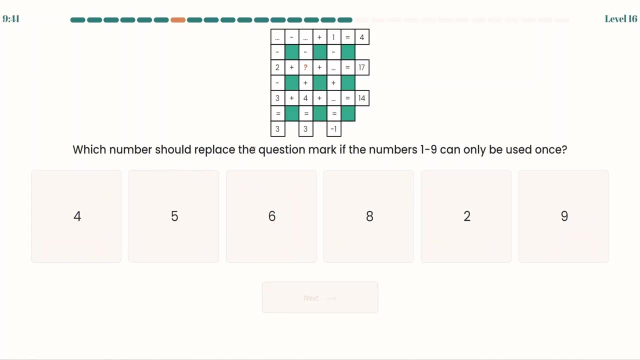 Oh, no, no, no, It's three, W, L, and then yeah, yeah, it's three. Which number should replace the question mark if the numbers one to nine can be only used once? So to find this one, we need to first find this one. three plus four, that's seven minus. 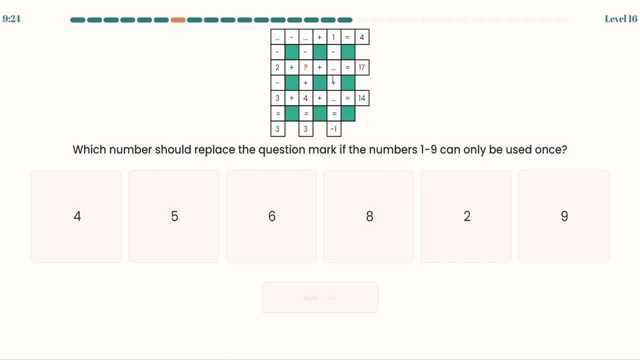 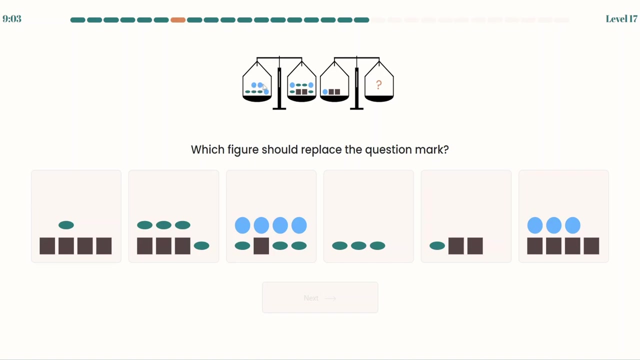 14, that's seven. Seven plus one, it's eight. Eight minus nine. Nine is minus one. this is nine, two plus nine. two plus nine is 11, then its question mark is six. Which figure should replace the question mark? 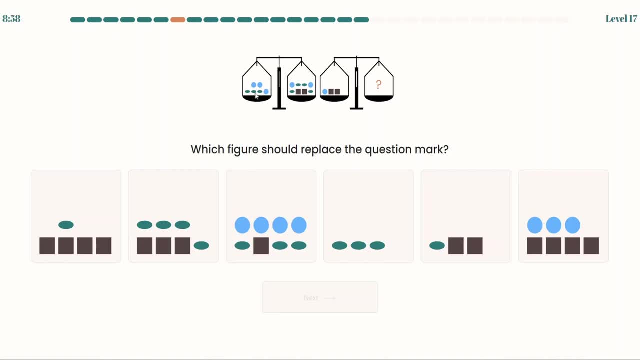 Three circles. we can eliminate two of them, and three blue dots. we can eliminate all of those. So one circle equals nine. One circle equals one blue dot and two black squares. One circle. one circle equals two black dots and one, two black squares and one blue dot. 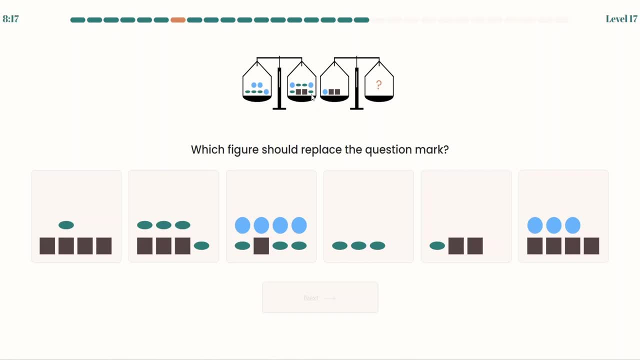 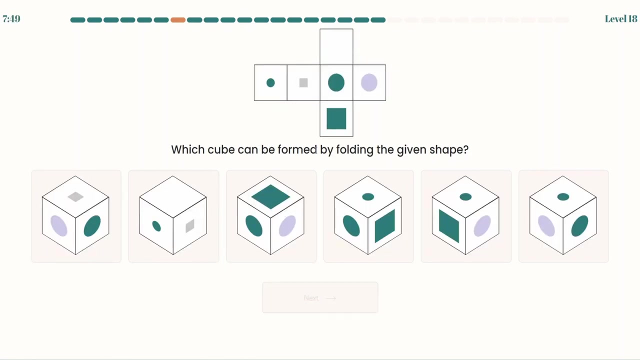 Blue dots, so we can pick, so we can move two over, so it's four of them. four black squares plus one circle. four black squares plus one dot- Yes, that's correct. Which cube can be formed by folding the given shape? 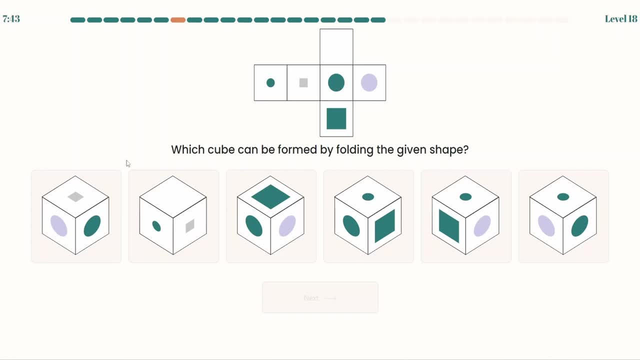 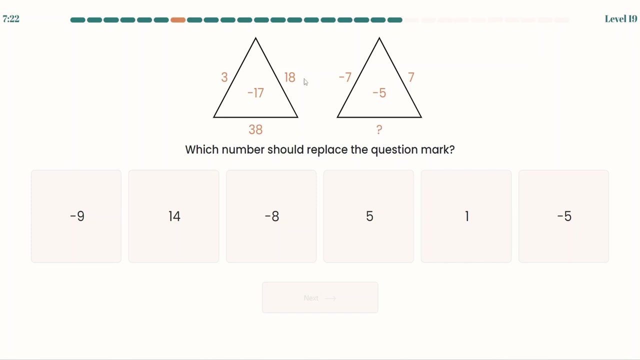 Is it this one? No, it's not this. Is it this, No, or is it? Wait, It's number two. Which number should replace the question mark? Three, Eighteen, Thirty-eight, Thirty-eight, Three, Three plus eighteen, that's twenty-one. 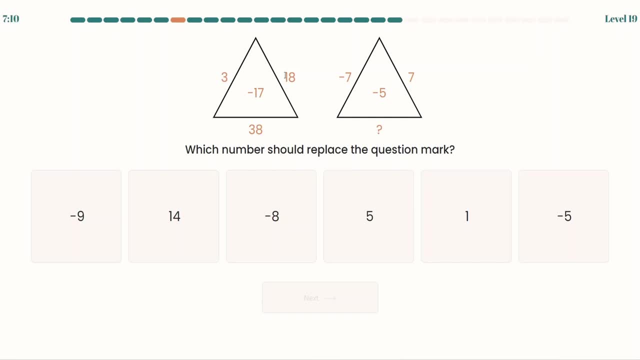 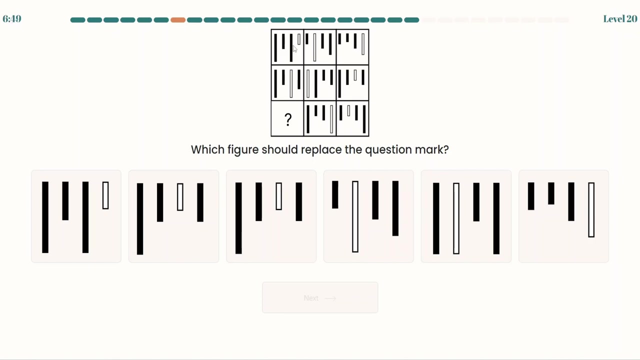 That plus that, minus that, so it's minus. wait, it's five. or is it wait minus that? is that? okay, it's five. Which figure should replace the question mark? Three, That, that, that? so it seems like wait what's? the one on the right side is growing. 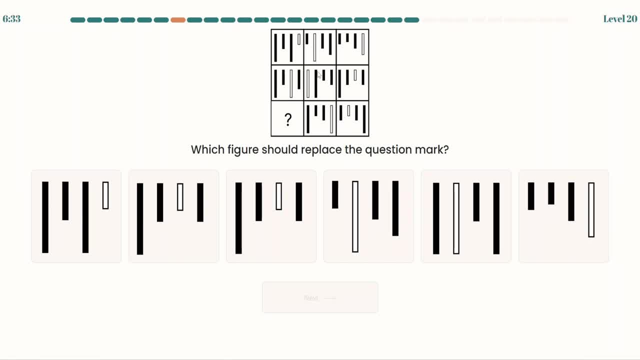 When you look downwards, we see that this one is moving to the left. And what's going on here? There's three white squares. This one, this, has three white squares. This is a square Moving to the left. this is really hard. I don't know what to expect here. 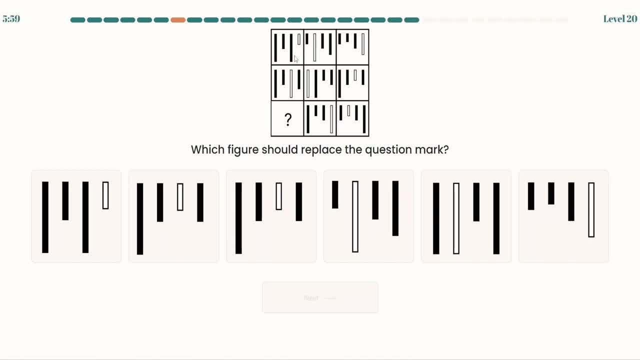 It seems like these three are conserved Because one area goes left. Okay, Okay, Okay, It pushes everything to the start. I mean, I guess it's this one. Oh, it was wrong. I need to look back at that one. 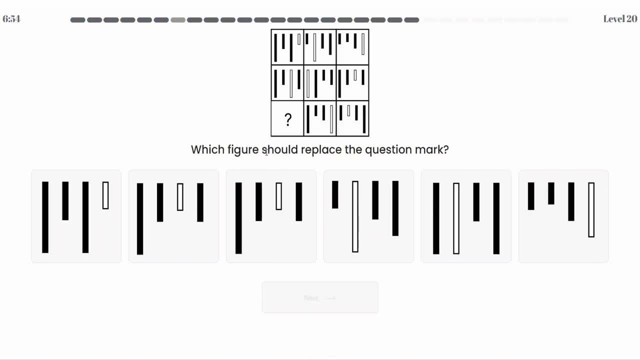 Okay, so this was the first puzzle that I don't understand. If we make all these lines the same length and then look at the columns, we see that the white lines moves one to the left, and if it's all the way to the left it reappears. 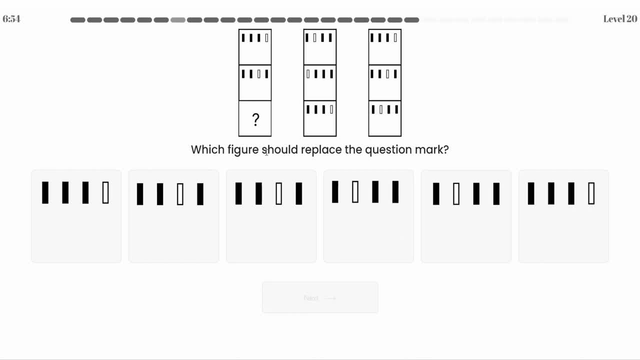 on the left. If we look at the first column, we see that the white line is at place number four, then three, and then it should be at place number two in the answer. This leaves only answer four and five. Now, when it comes to the lengths, I really have no idea how they work. 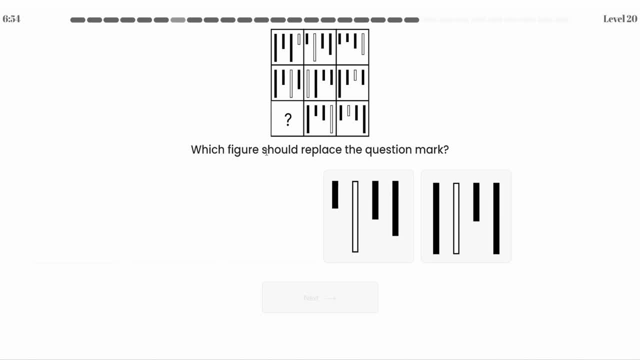 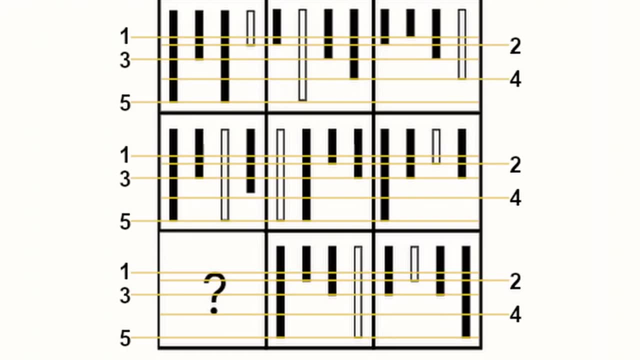 At first I thought there was only four different lengths. However, when I zoomed in, I realized that there was five different lengths And after I made this overlay, I realized that there was six different lengths. I have no idea how these pictures are related. 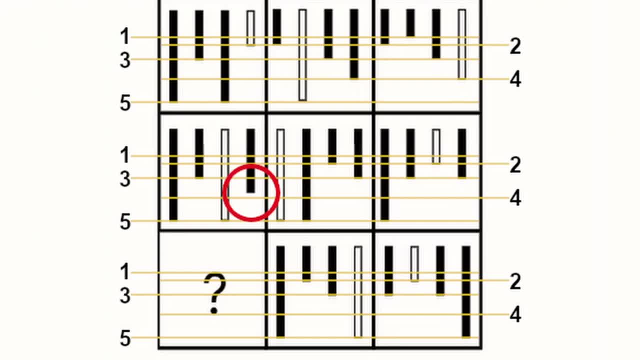 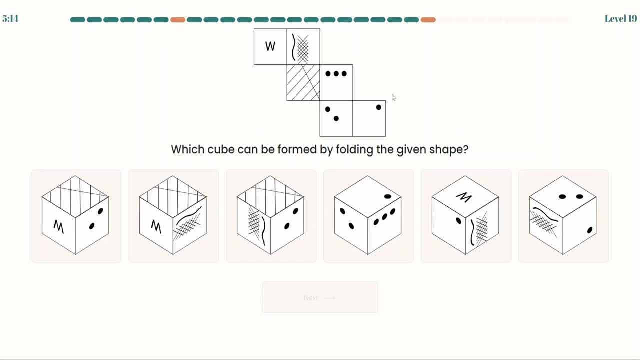 If you understand this puzzle, please let us know in the comments how it works. Which cube can be formed by following the given shape W? Is it this one? No, because that line wait. is it this one? Yeah, it is. 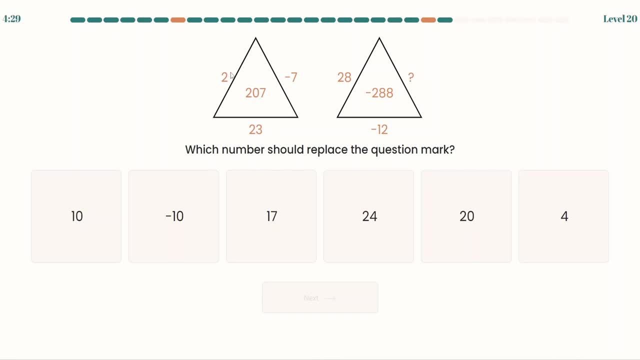 It is this one. It is this one. Yeah, it is. No, it is this one. This is the one. No, it is this one, No the other one. I could have done the other way around, Maybe, but I can't think of it. 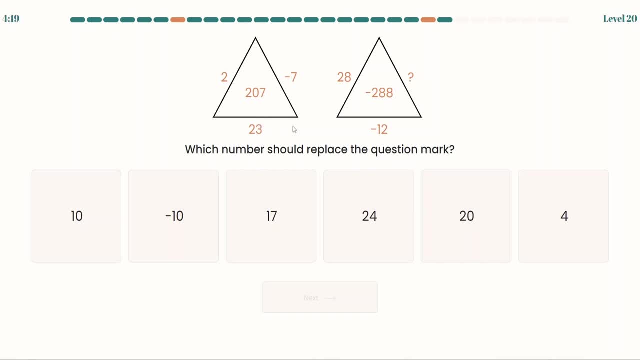 So that one is there. that one is. that one is All right. Well, let's go ahead and get the second one. So that one here. this is the first one. That one is the second one. I have to find the first one right. 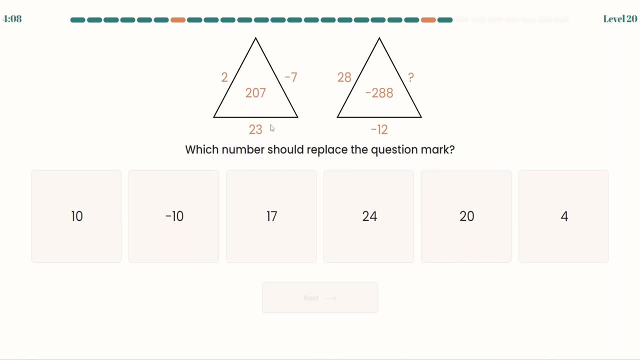 I want to get the second one again, So I'm going to write this one. I don't want to write the first one, so I'm going to write this one: 140 plus 21,, that's 161, 23 squared. no, that can't be it. 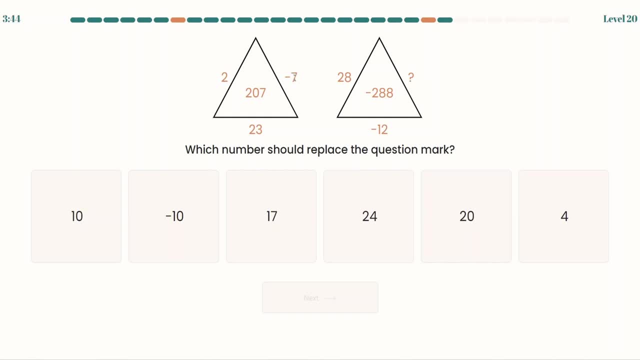 26,, 27,, 28,. hmm, which number should replace the question mark 23.. 23 times 7,, that was 140 plus 21,, 161,. so it's not multiplication of those 23 squared. 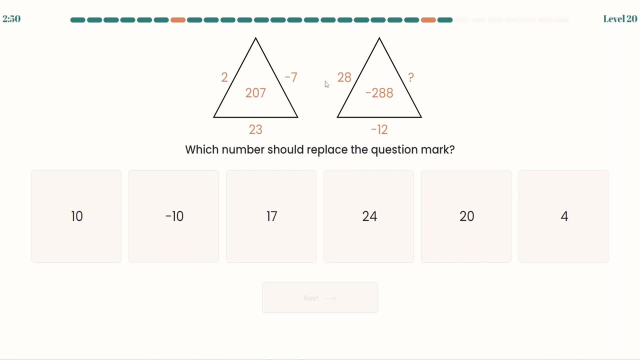 oh, I don't really know. it looks like the 7 goes there. it can't be. I feel like it has to be 4, maybe, Or 10, because 10 is twice, hmm, 280,. since this is negative, it has to be minus 10, oh. 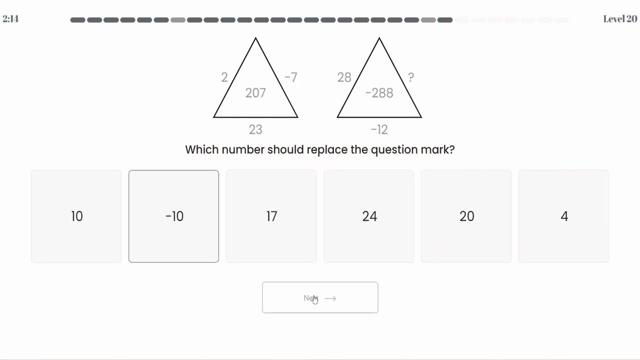 that was wrong. I have to look back at that. Looking back at this problem. it was actually quite easy. so first I took 207, divided it by 23 to get 9. And I realized that 2 minus minus 7 is equal to 9.. 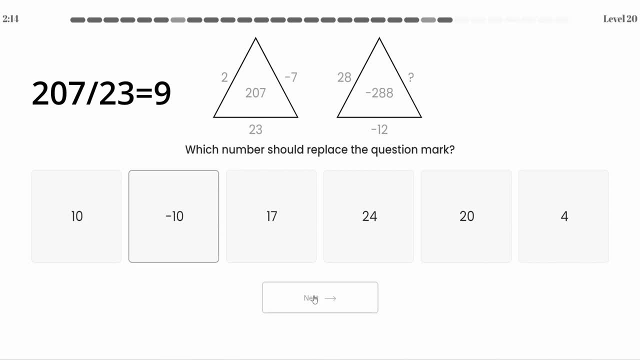 So to get the number in the middle of the triangle, we take the top left minus the top right and then multiply it by the number under the triangle. To solve this puzzle, I took minus 288,, divided it by minus 12 to get 24,. 28 minus 24 is 4,. 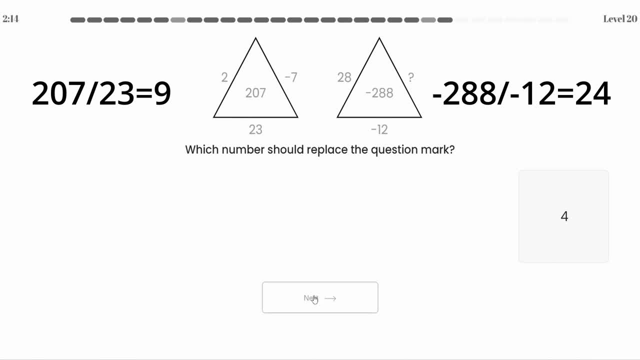 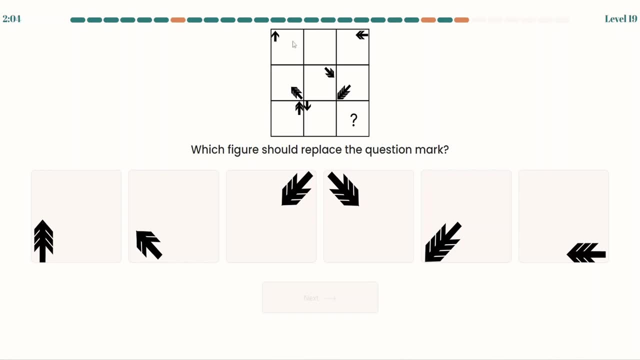 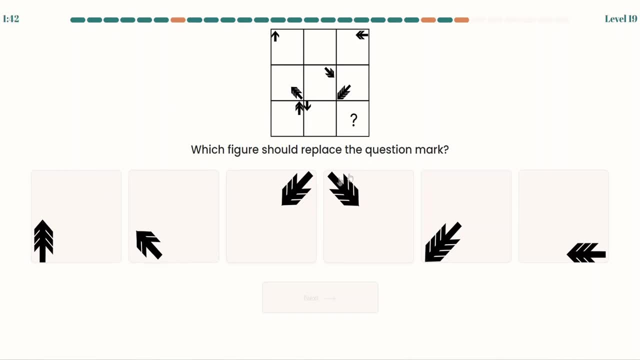 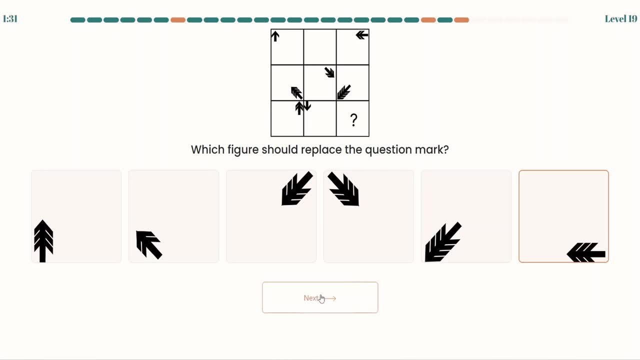 I mean, this has already appeared, so I'm guessing it's 6, yeah, that's an easy one. Which 3 shapes can be combined to create the figure on the left? Hmm, I don't know. I don't know. 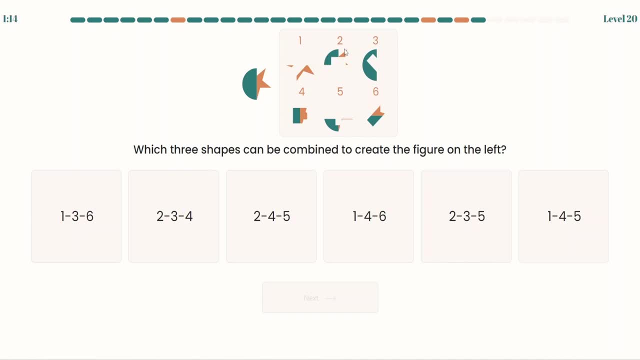 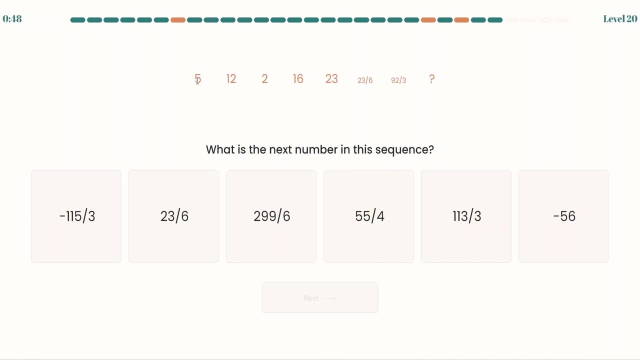 So increase, decrease, Increase, decrease, Increase, Increase, Decrease, Increase, Decrease, Decrease, Decrease, Decrease, Decrease. This is a really hard one as well. So 5 to 12 plus 7 minus 10, or divided by 6, multiplied by 8, increase, decrease, increase. 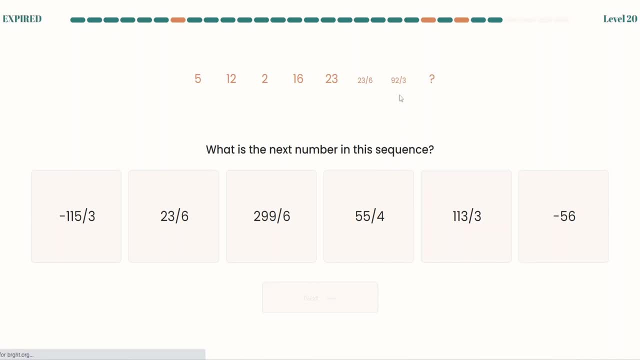 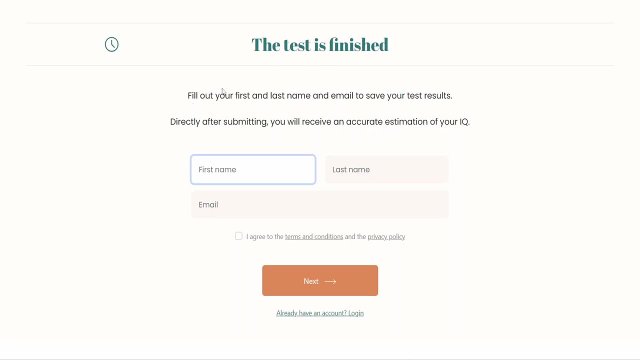 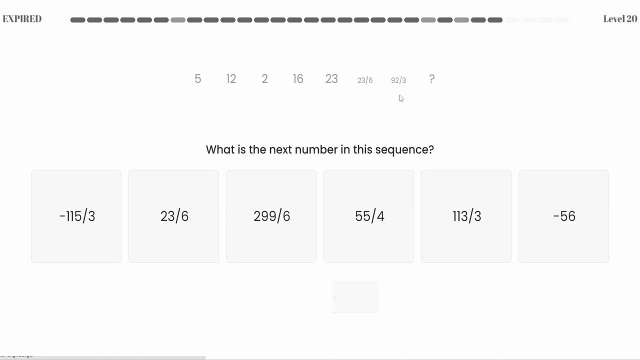 increase, decrease, decrease. yeah, that was it. Uh, the test doesn't give me an instant score, so I guess I have to make an account and we will see Before looking at the score. I just want to quickly explain this puzzle. 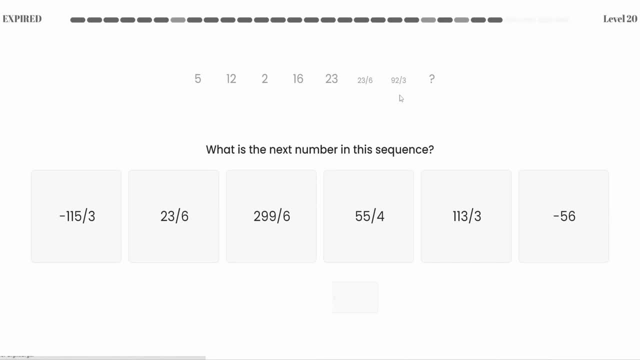 So we have the sequence 5,, 12,, 2,, 16,, 23,, 23 divided by 6,, 32 divided by 3, and question mark. So first we take plus 7,. 5 plus 7 is 12.. 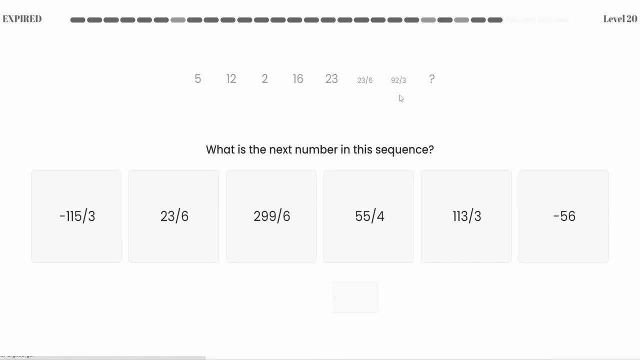 Then we divide by 6,: 12 divided by 6 is 2.. Then we multiply by 8,: 2 multiplied by 8 is 16.. Then again we add 7, 16 plus 7 is 23.. Then we divide by 6,: 23 divided by 6 is 23 divided by 6.. 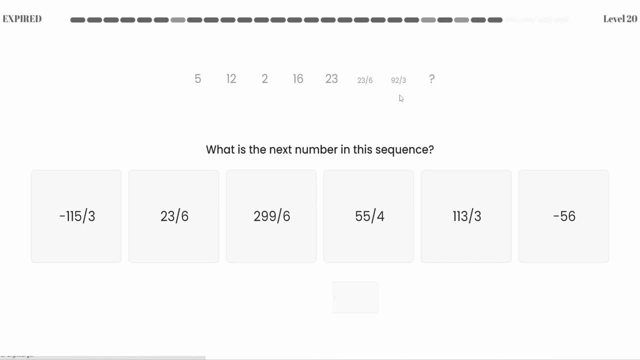 And then we multiply by 8, 23 divided by 6 multiplied by 8 is 92 divided by 3.. And at last we add 7.. So we have 92 divided by 3 plus 7. That's the same as 92 divided by 3 plus 21 divided by 3.. 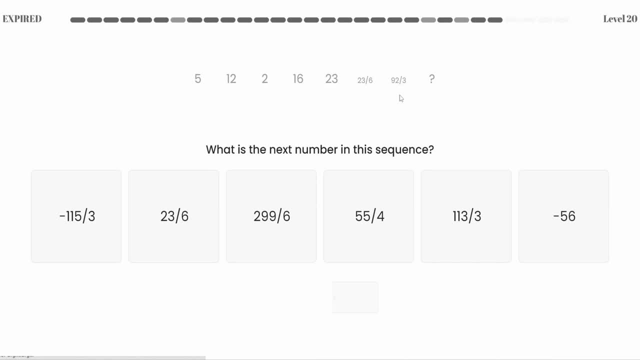 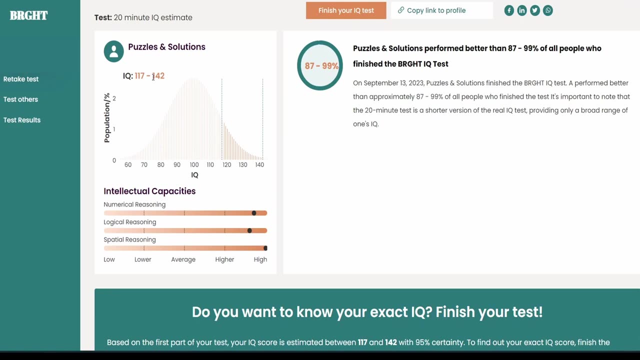 So the answer is 92 plus 21,, 113 divided by 3.. Answer number 5 is correct. So here is my final score: I got a range from 117 to 118.. So I got a range from 117 to 118.. 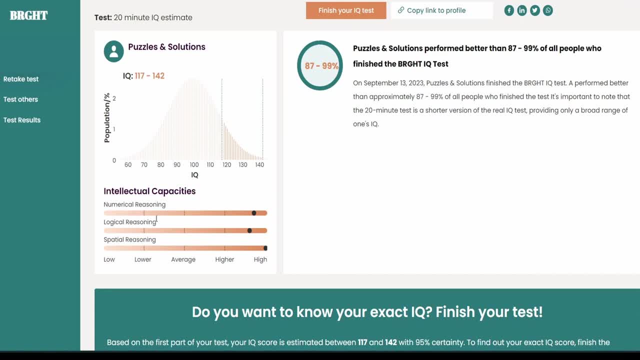 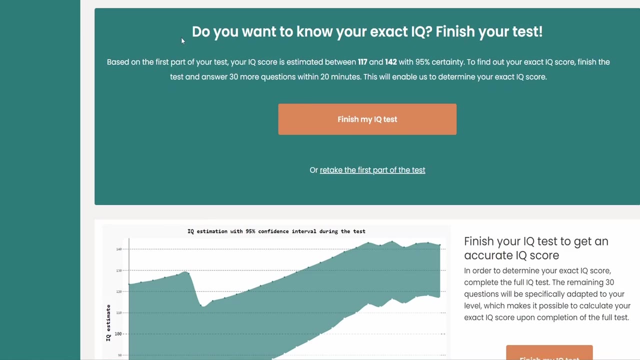 It seems like my numerical reasoning, logical reasoning and spatial reasoning were all high. And it says puzzles and solutions performed better than 87 to 99% of all people who finished the bright IQ test. And further down on the page it says: do you want to know your exact IQ? 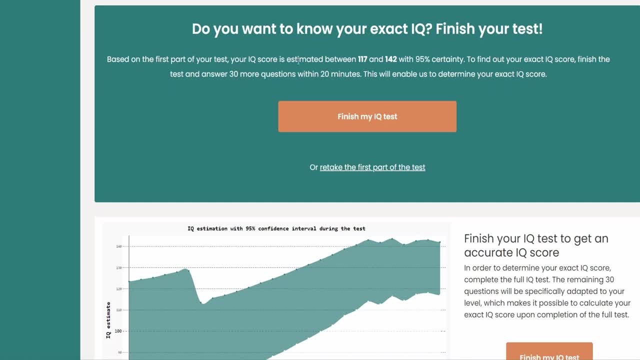 Finish your test. Based on the first part of your test, your IQ score is estimated between 117 and 142. with 95% certainty, Answer number 6 is correct. It seems like my numerical reasoning, logical reasoning and spatial reasoning were all high. 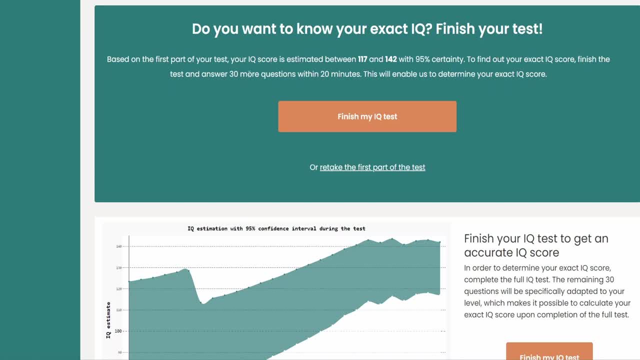 It seems like my numerical reasoning, logical reasoning and spatial reasoning were all high. And further down on the page it says: do you want to know your exact IQ? Finish your test. Based on the first part of your test, your IQ score is estimated between 117 and 142 with. 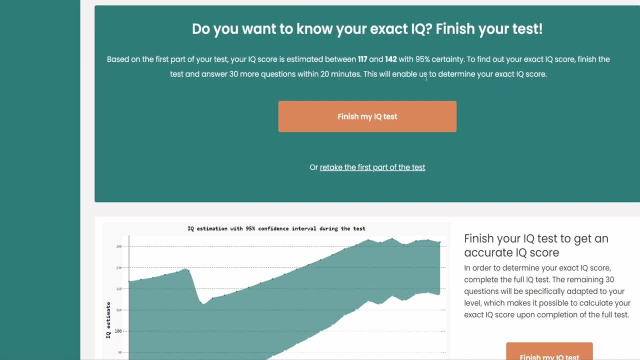 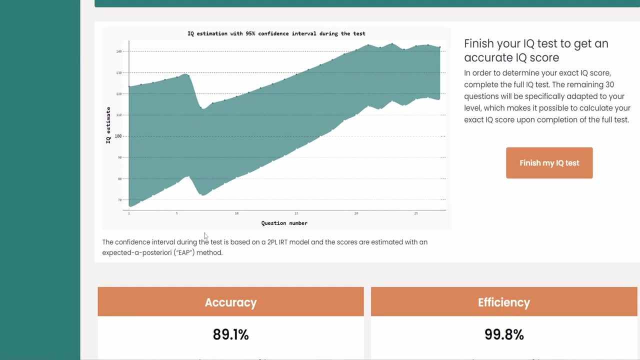 95% certainty. To find out your exact IQ, finish the test and answer 30 more questions within 20 minutes. This will enable us to determine your exact IQ And here we see an IQ estimate over time or the questions answered. So at first it starts from it seems like 65 to 125, and then over time it increases the value. And at the last it was between 117 and 142.. Finish your IQ test to get an accurate IQ score. In order to determine your exact IQ score, complete the full IQ test. The remaining 30 questions will be specifically adapted to your level, which makes it possible. 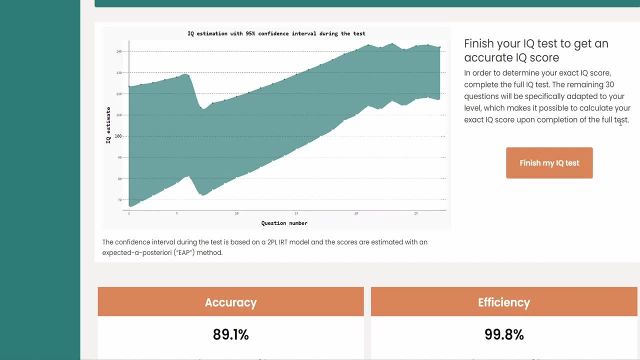 to calculate your exact IQ upon completion of the full test. That was everything for today. I might finish the IQ test In the future. let me know if you want to see more of this bright IQ test. I think it's really fun and it's a really good designed website, at least. 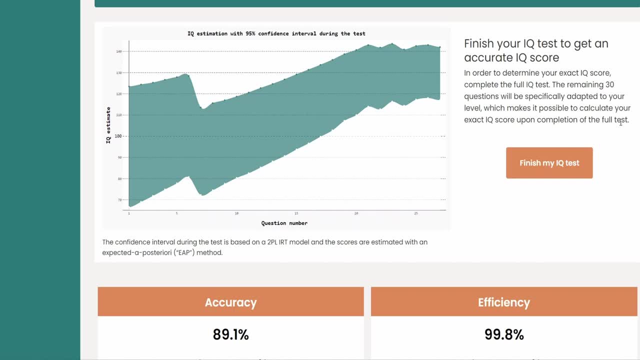 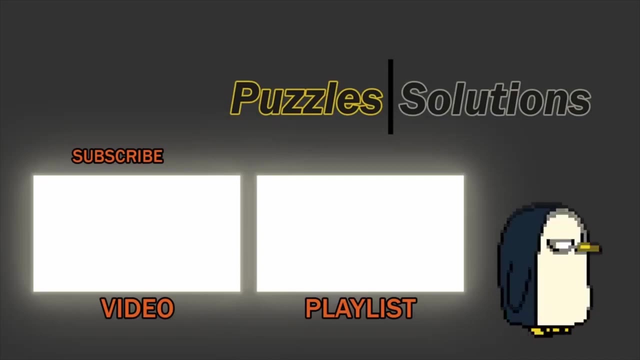 I don't know if it's a good design. IQ test: I feel like many of the questions I have to actually think. So, yeah, I kind of enjoy it, but yeah, that was everything. See you another time, Bye, bye, Bye.